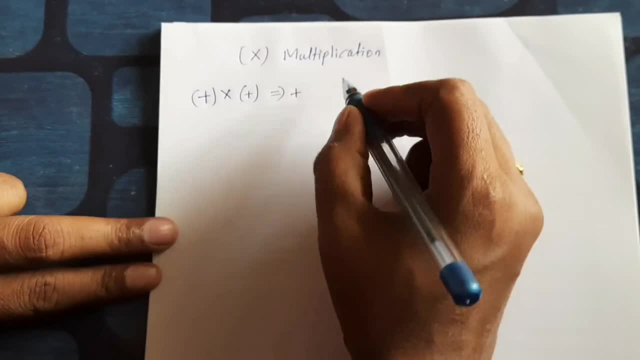 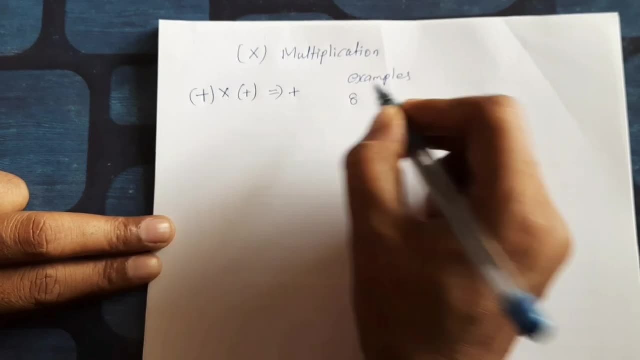 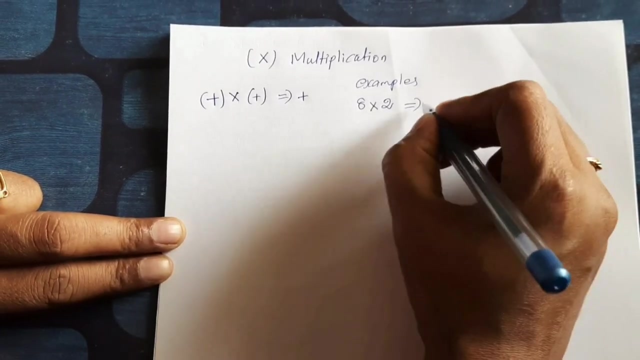 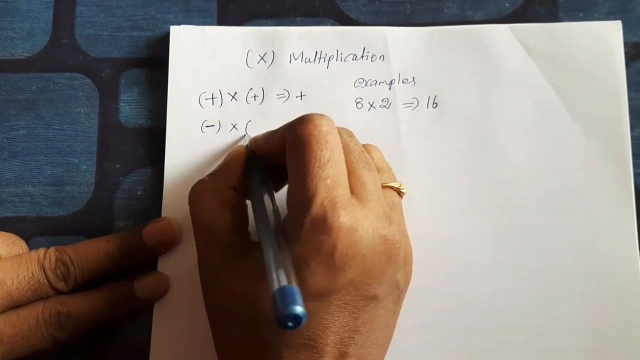 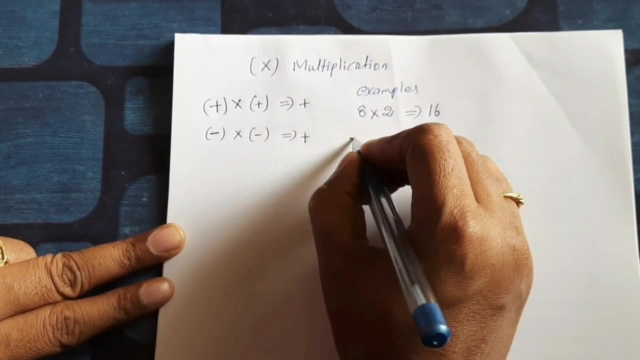 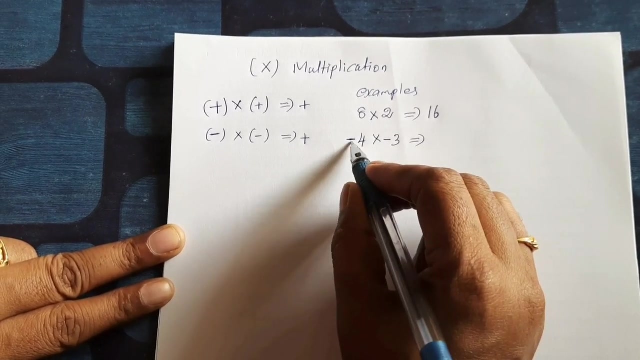 Minus gives plus. Examples: 8 plus 8 into plus 2, equal to 16, plus 16.. Now, minus into minus gives plus Example: minus 4 into minus 3 gives minus into minus plus 4 into 3, 12.. 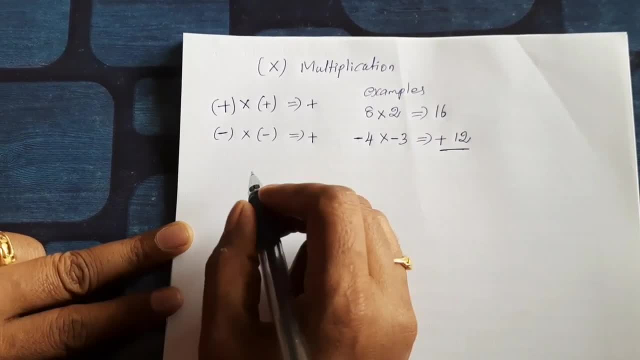 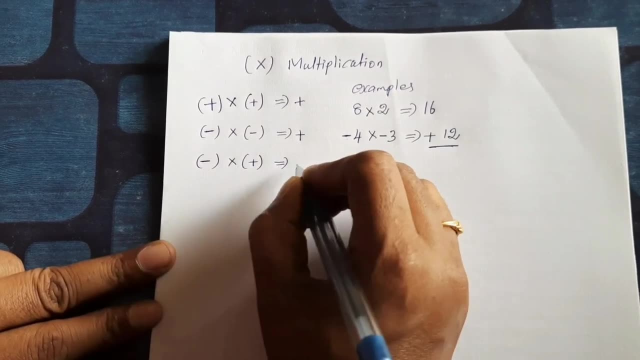 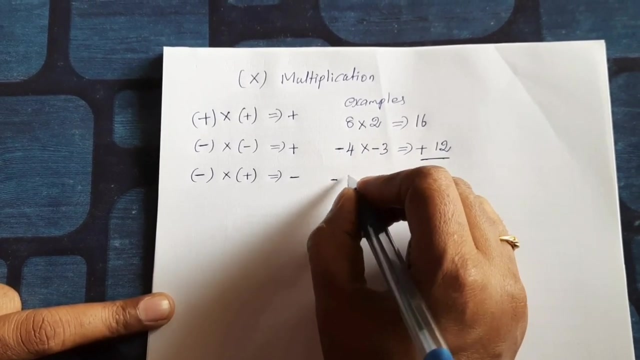 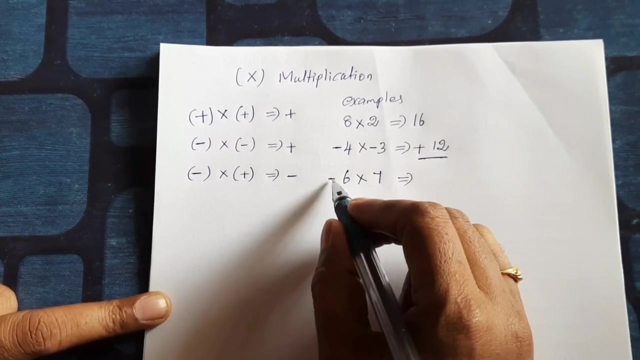 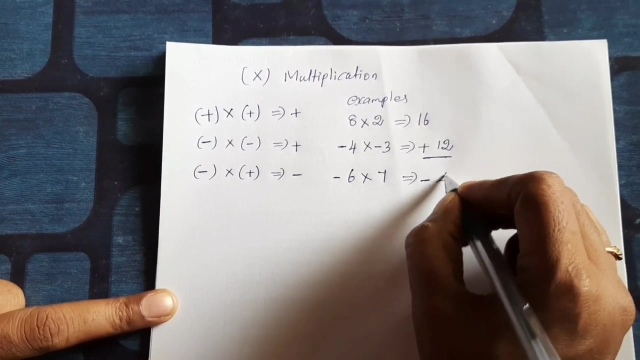 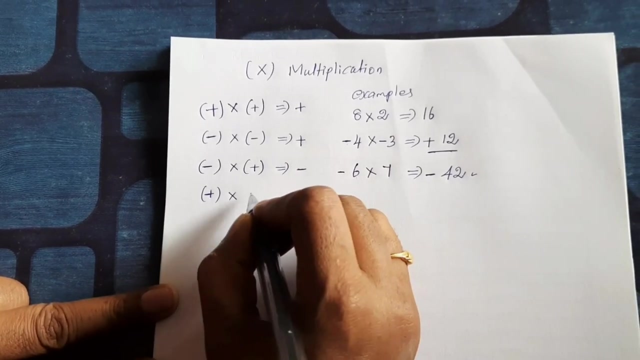 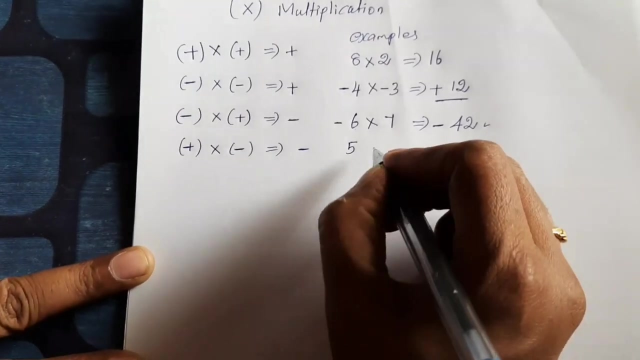 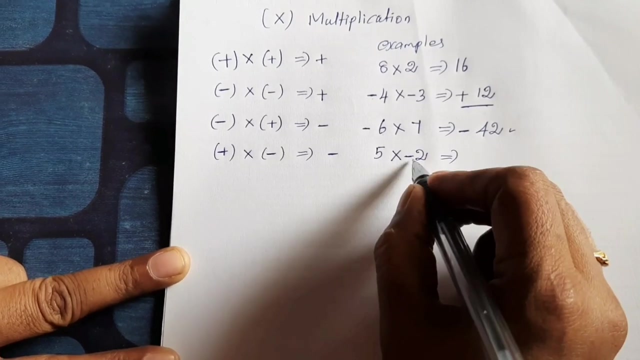 Next: minus into plus gives minus Example: minus 6 into plus 7 equal to minus into plus. minus 6 into 7, 42.. Next, plus, both are same. plus into minus gives minus Now 5 into negative. 2 equal to minus into plus. minus 5 into 2, 10.. 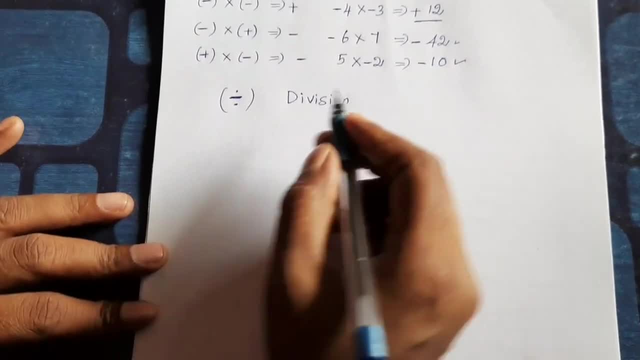 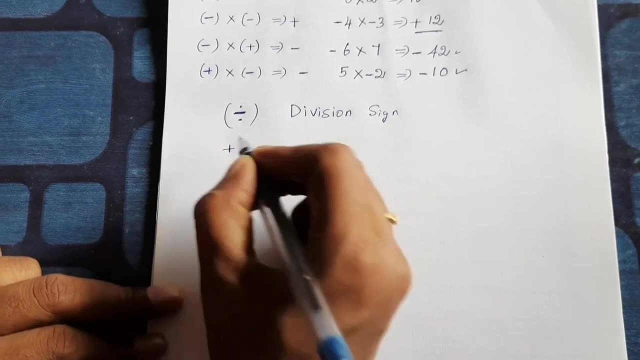 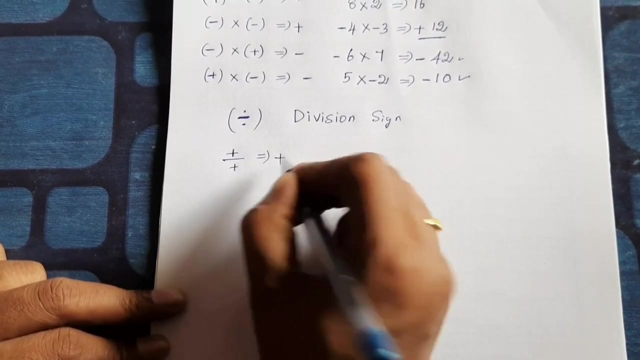 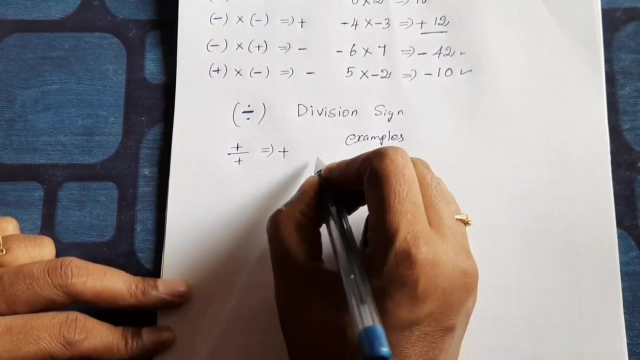 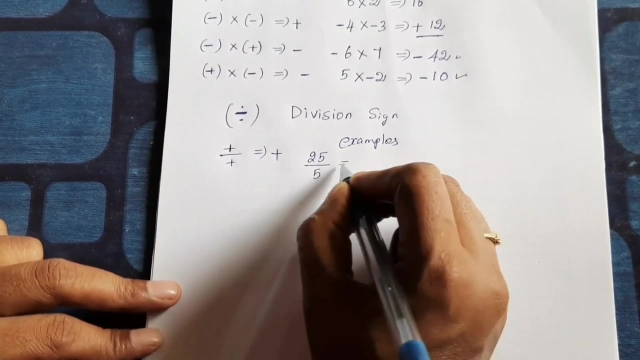 Next division sign. So plus divided by plus Next division sign. So plus divided by plus gives plus plus sign. So for example: plus 25 divided by plus 5 equal to 1 5sar, 5 5sar. 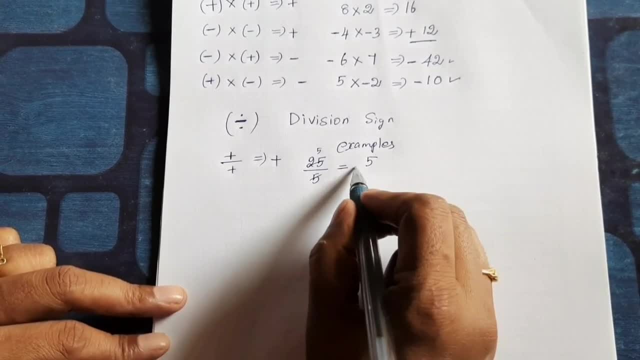 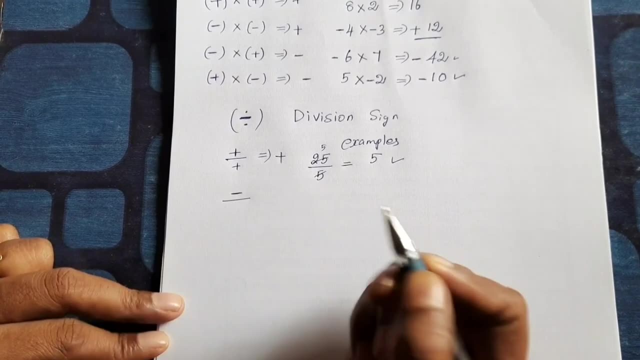 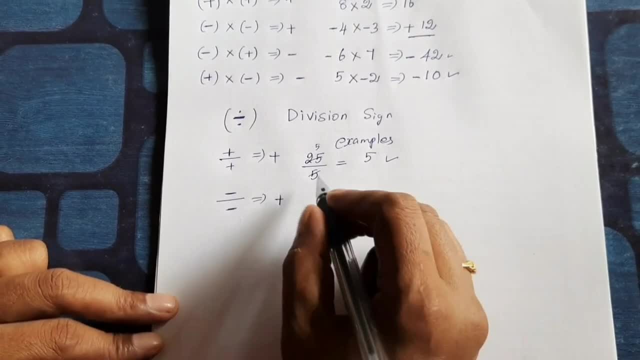 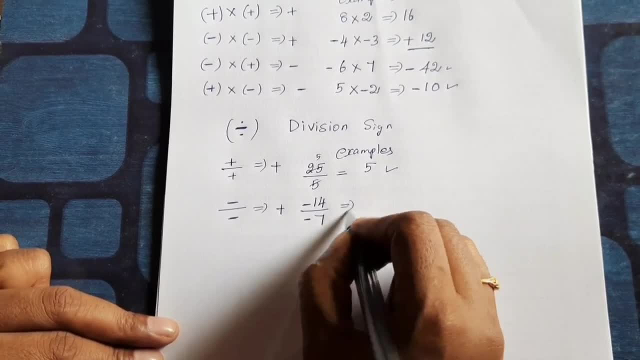 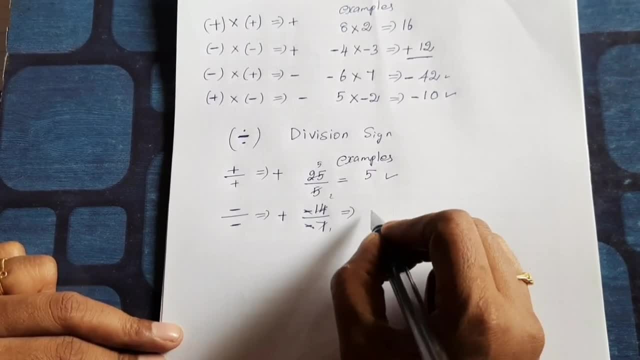 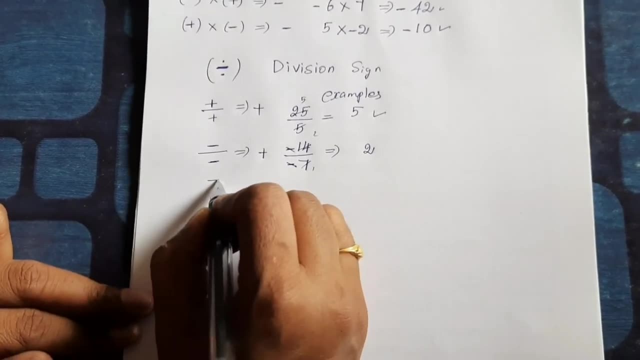 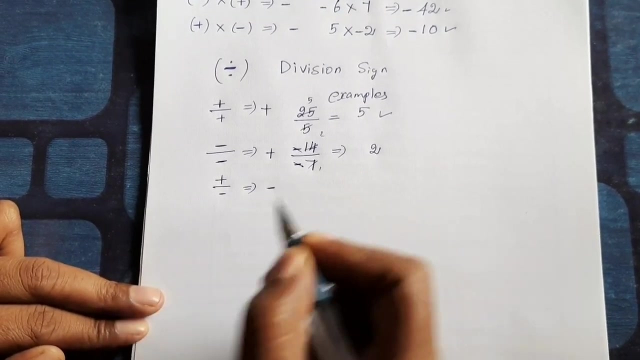 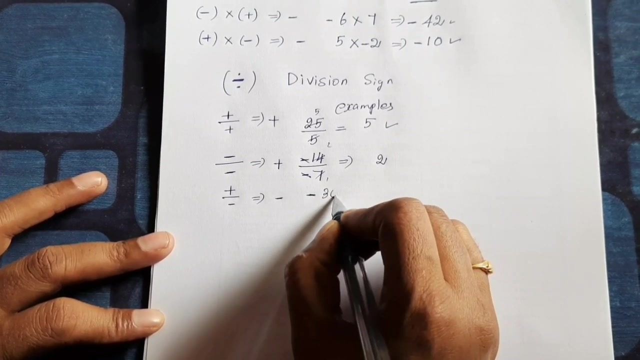 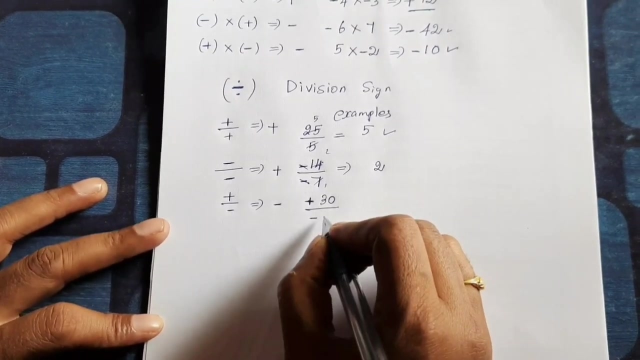 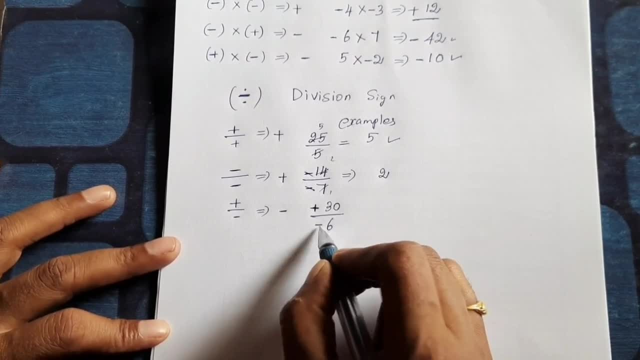 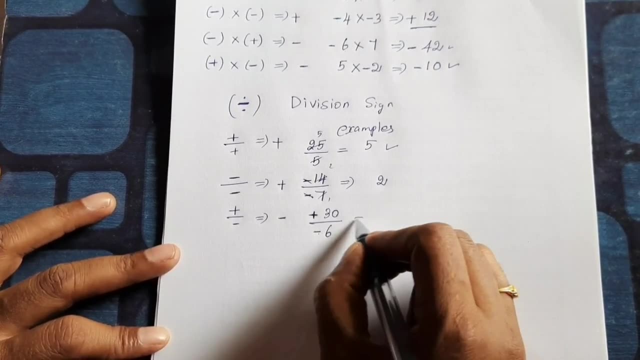 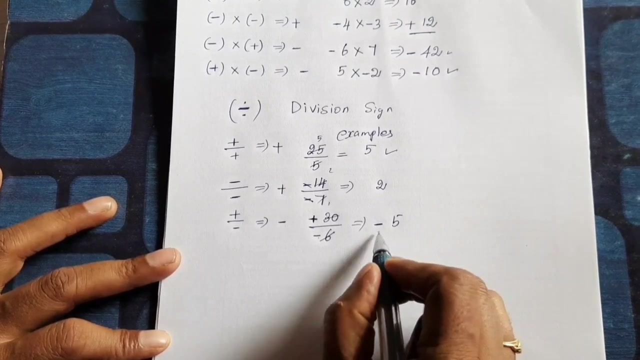 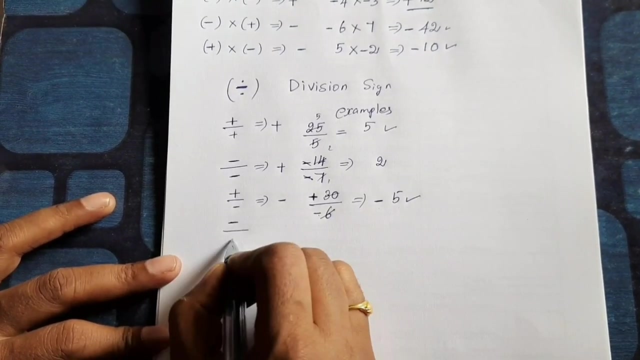 So denominator numerator any places negative signs, that is speaking common signs, common minus 1, 6er, 5, 6er, So negative 5.. Next, minus divided by plus gives same thing negative. 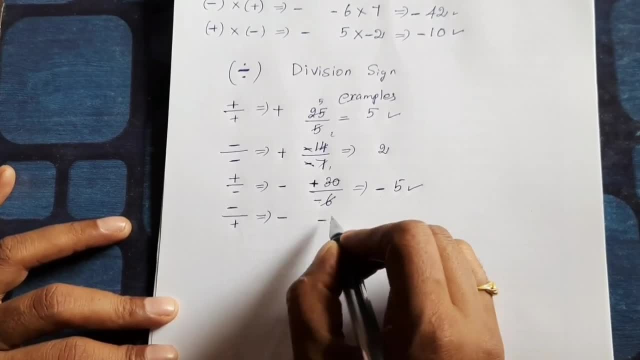 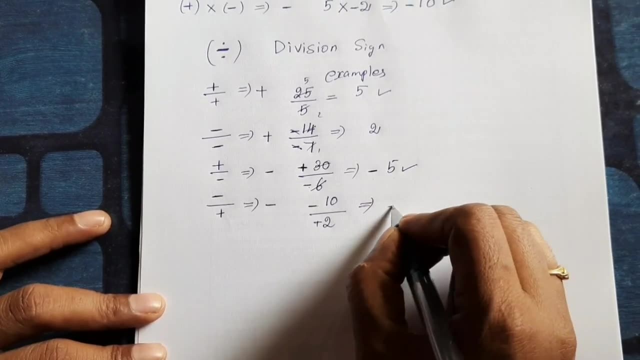 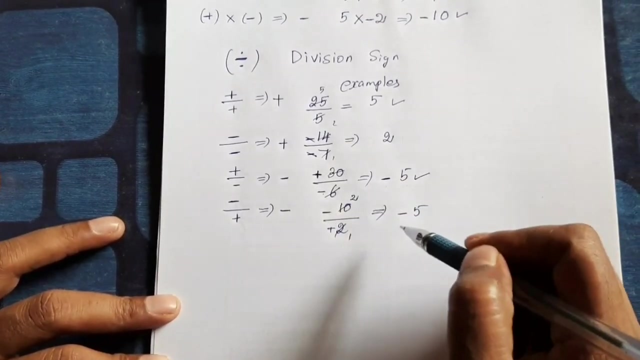 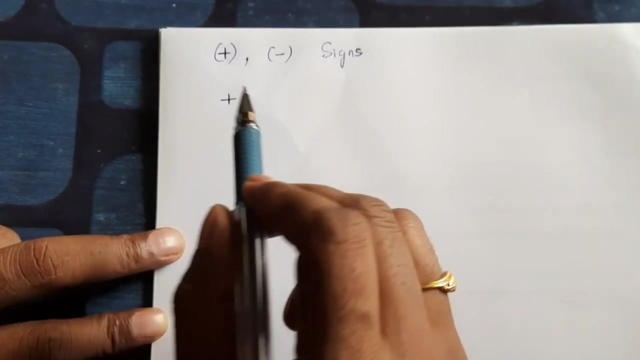 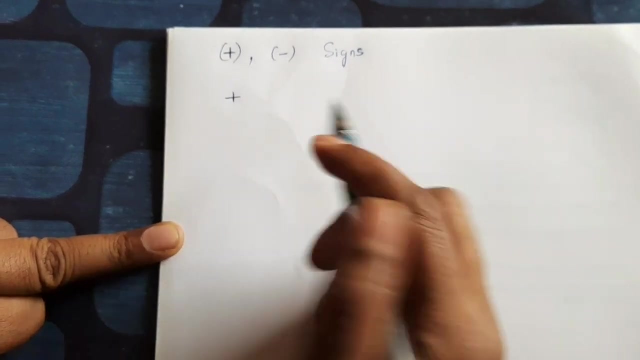 So minus 10 divided by plus 2 gives negative 5.. 1 6er, 2 6er. So understood this concept. Sorry, students, this is very, very important concept. Students making more mistake Here. so plus and minus sign. 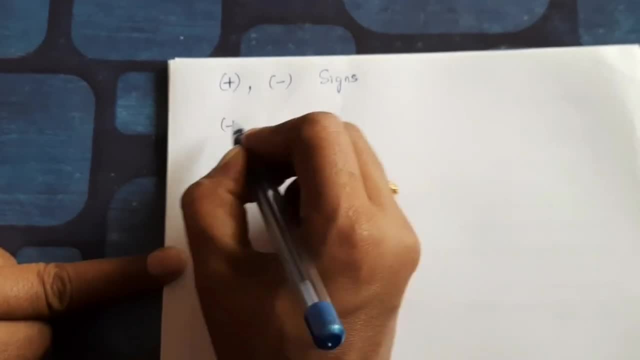 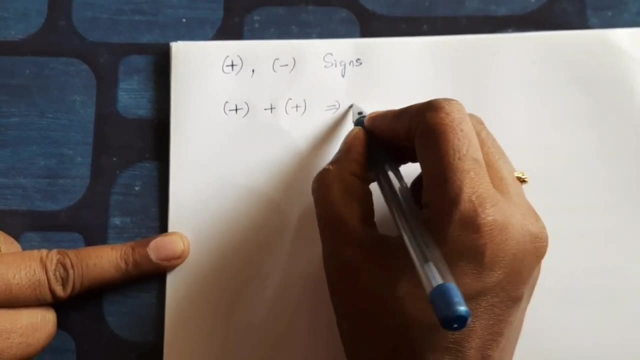 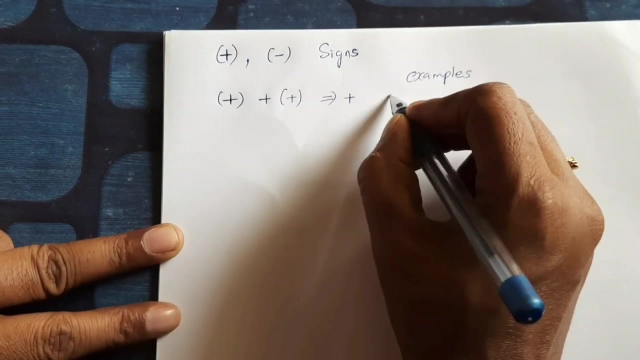 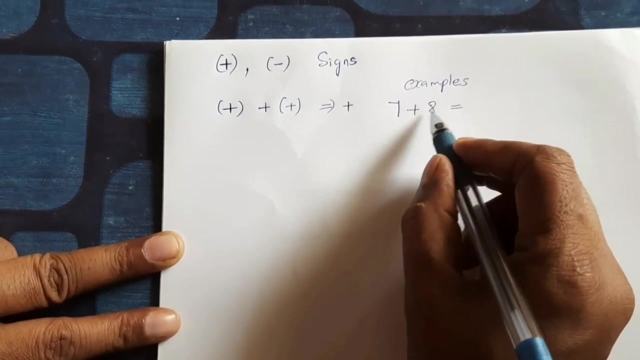 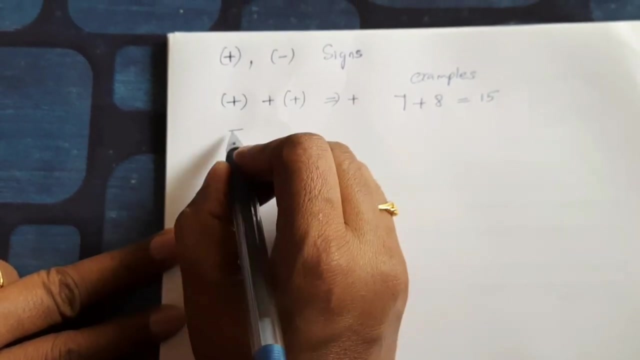 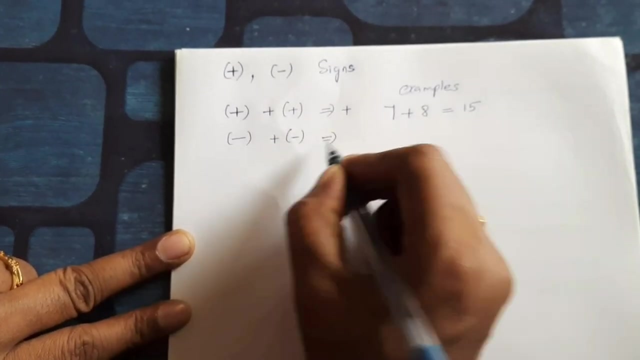 Here first plus sign: Plus, plus plus equal to plus. Example 7, plus 7, plus plus 8 equal to plus 50.. Next: minus plus minus, Minus. plus minus gives minus. 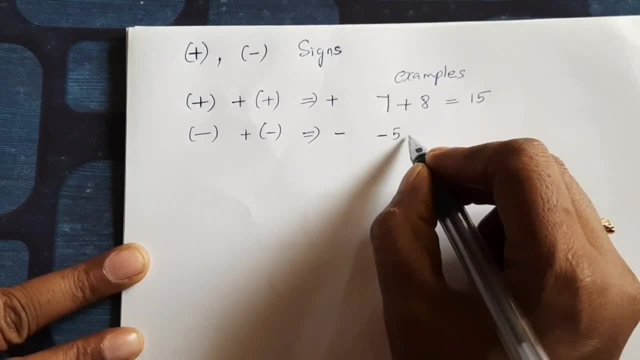 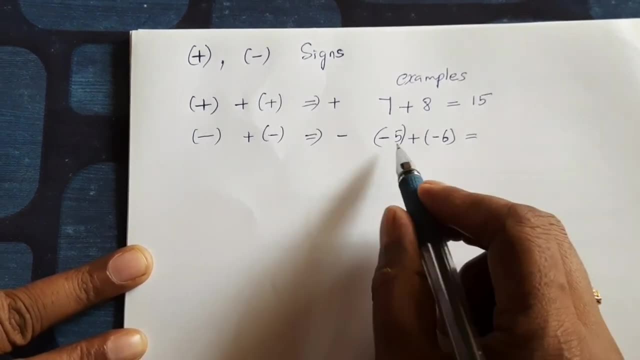 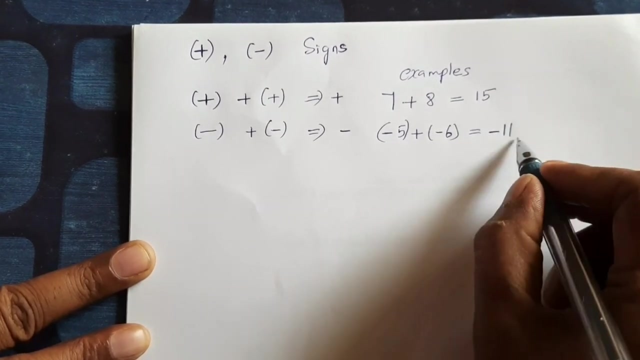 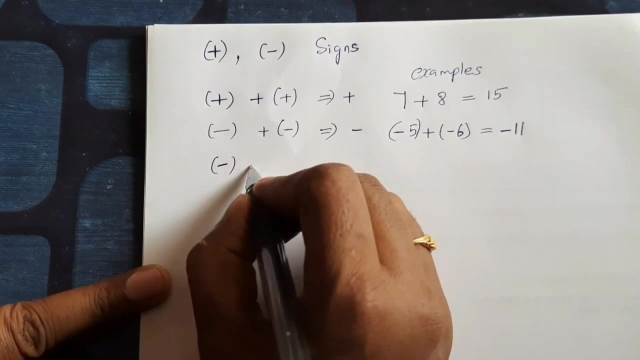 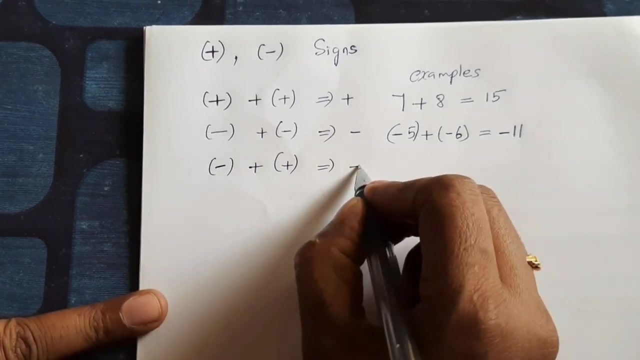 Here: minus 5, plus minus 6 gives minus, minus. minus 5 plus 6 less 11,, so negative 11,, not plus 11.. Next, minus plus plus It gives minus. This is very, very important thing. 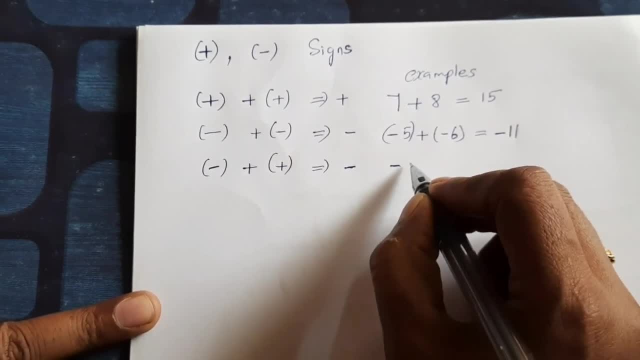 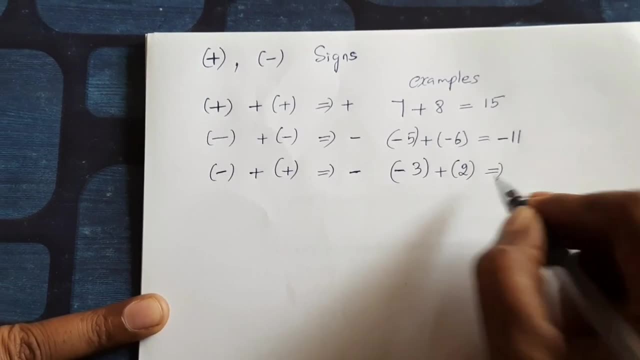 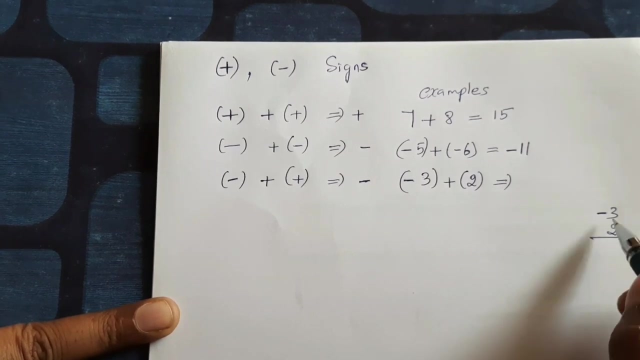 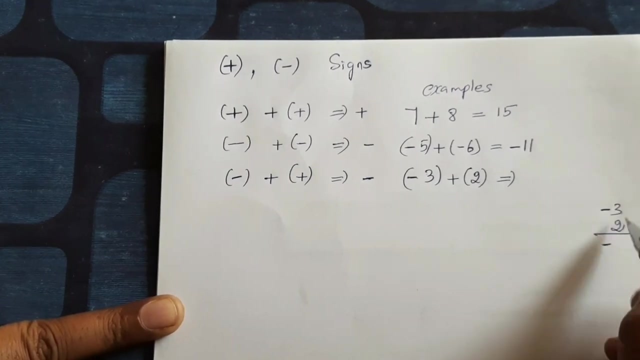 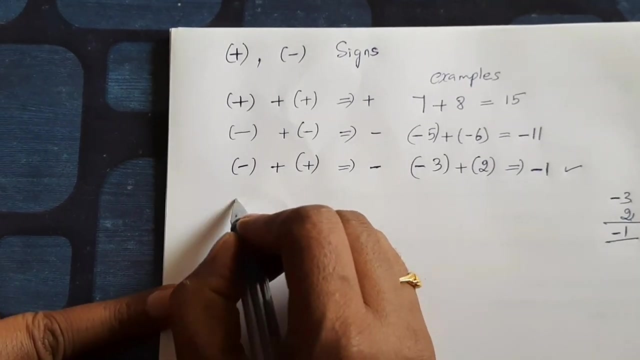 Suppose: minus 3 plus 2. It gives minus minus 3 plus 2. So negative sign is highest value. So we put negative sign 3 minus 2,, 1. So minus 1.. Next: plus plus minus. 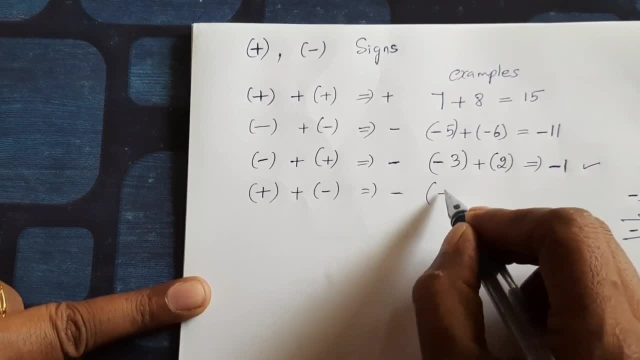 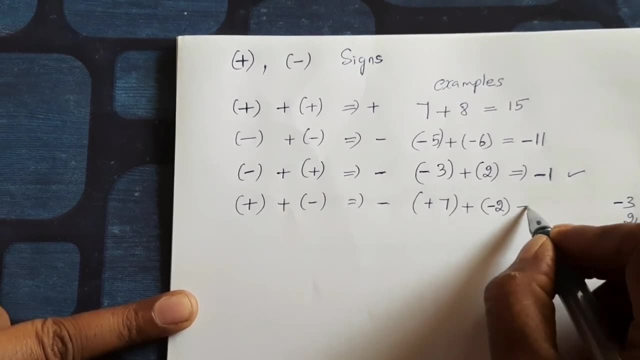 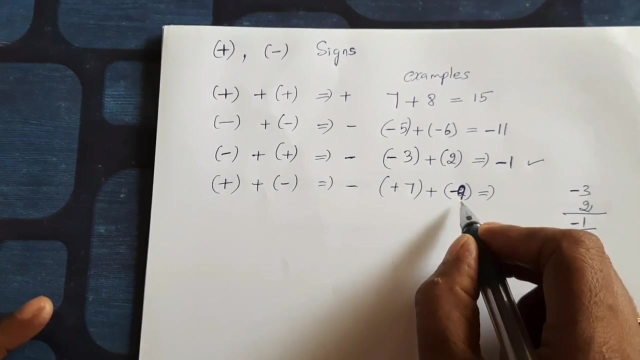 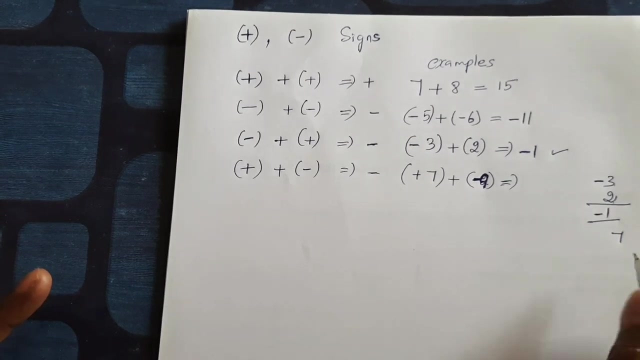 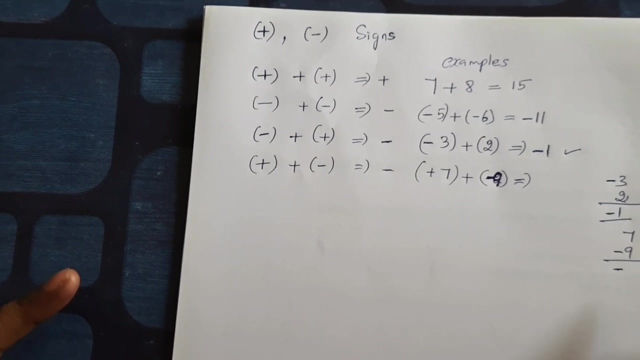 It gives negative. So plus plus minus. So plus 7, plus minus 2. Minus 9. So it gives: 7 is positive number, minus 9 is negative number. So here also negative sign is highest. 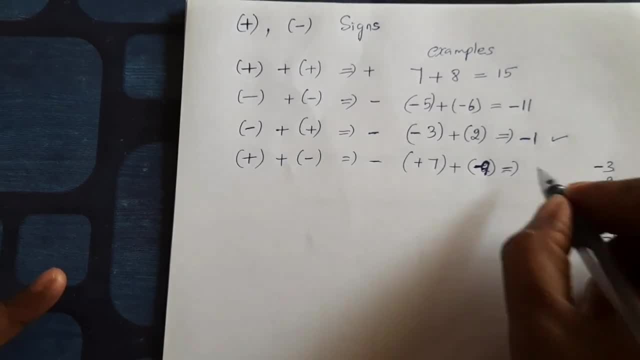 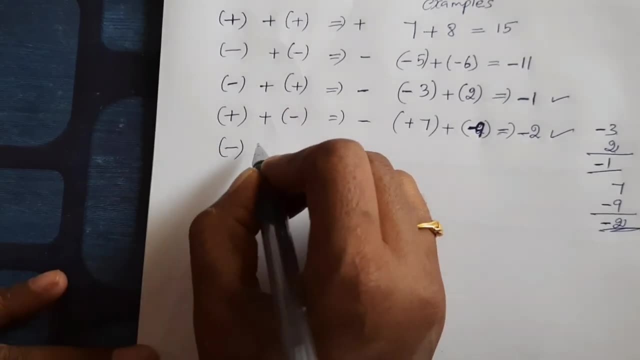 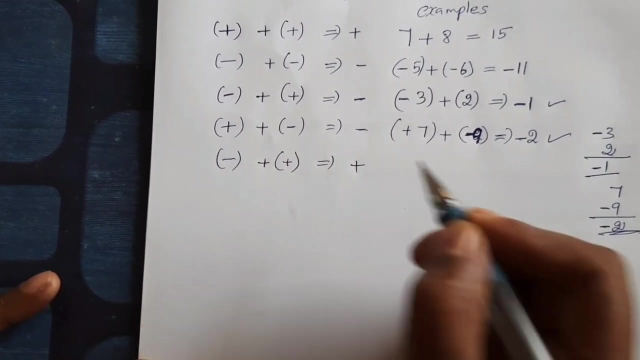 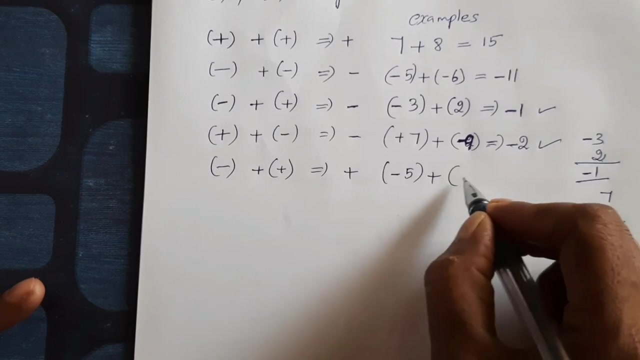 Plus. that is what Minus 2., So minus 2.. Same thing next: Minus plus plus. It gives plus. because here suppose minus 5, plus is plus, value is more than 5. So 10.. 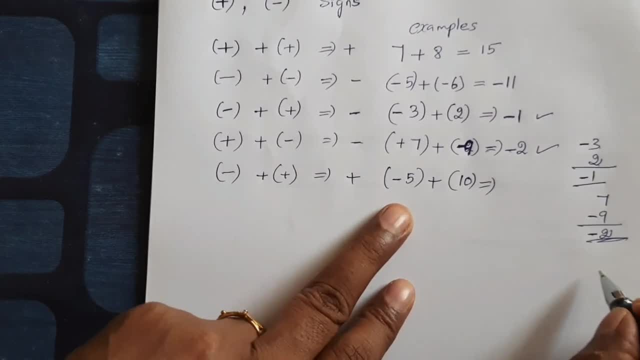 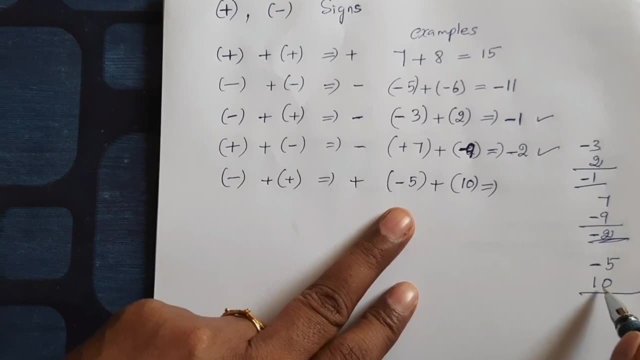 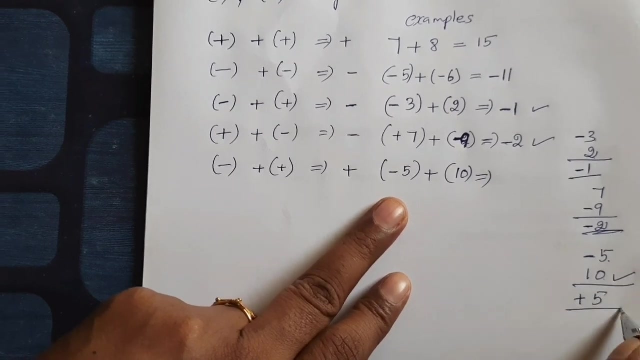 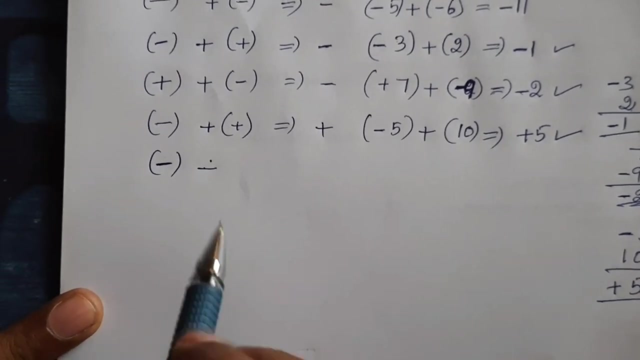 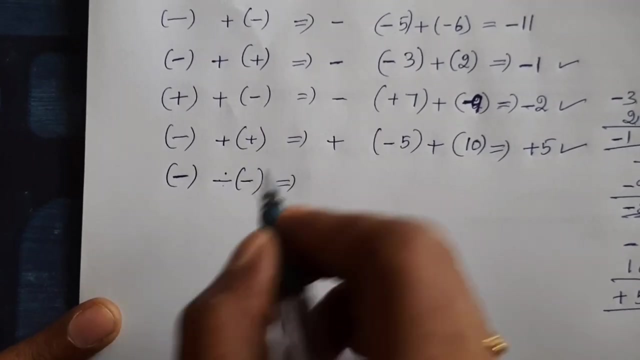 You take 10. So minus 5, positive 10. Now which sign is highest? Positive sign is the highest, So plus sign. So 10 minus 5 is positive 5., Plus 5.. If your student have some same doubt, I will clear now. So minus, minus, minus Equal to what Minus. 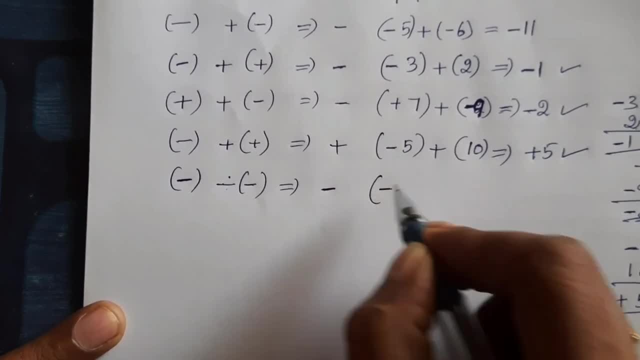 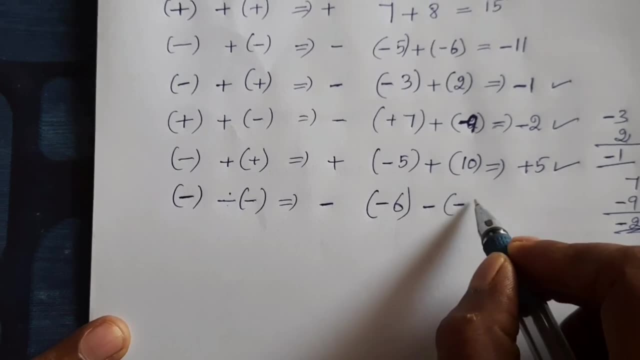 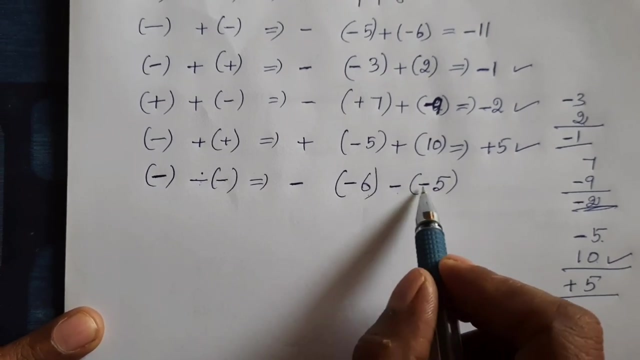 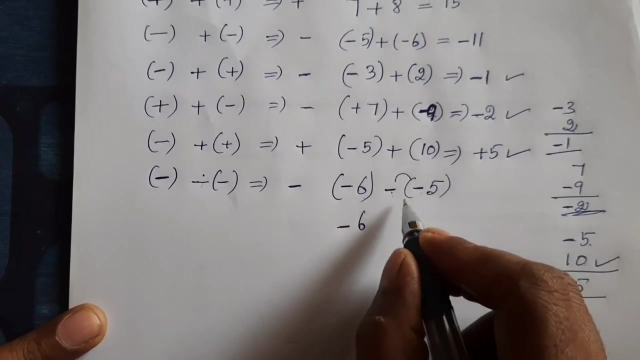 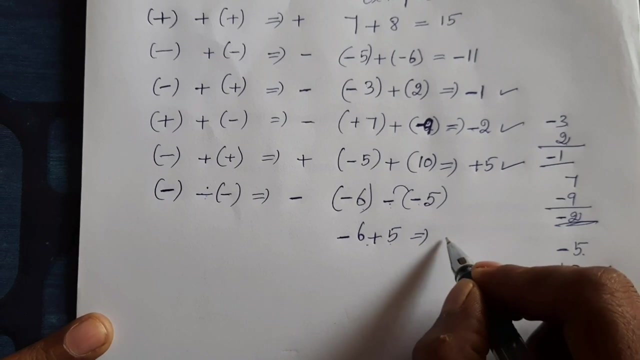 So my example: minus 6, minus minus 5.. Now minus 6, minus of minus. So it gives, suppose minus 6, minus into minus What Plus, So plus 5.. Equal to now minus 6, plus 5.. It gives what Minus 1.. That is small number, So get positive number. 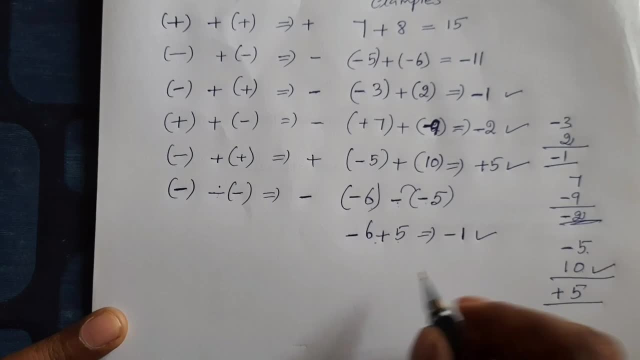 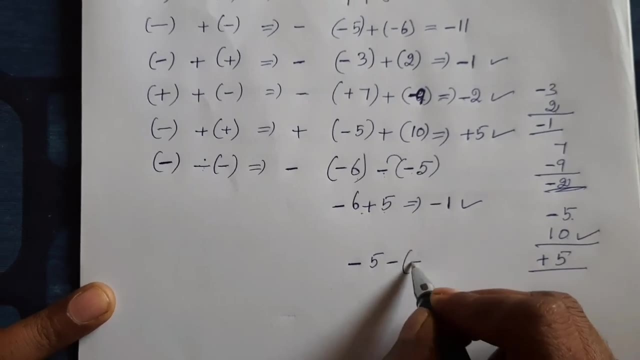 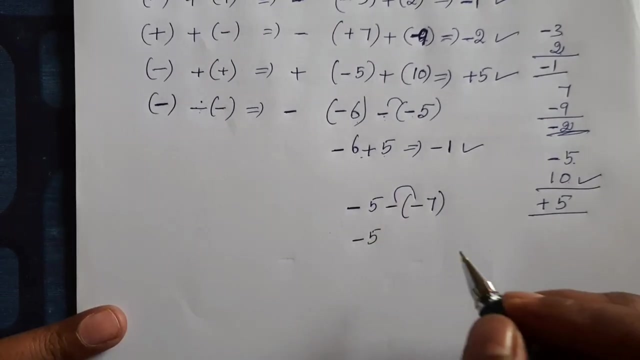 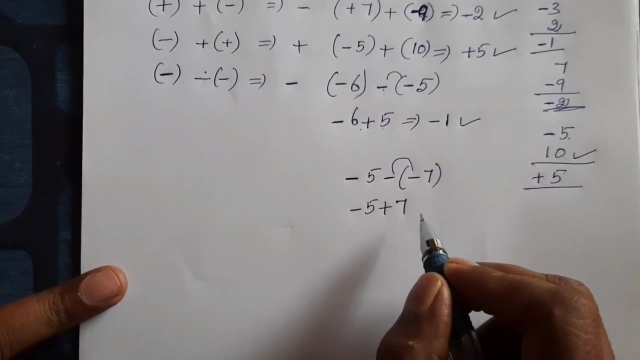 Now one more example. So minus 5, minus Of minus 7. It gives minus 5, minus into minus plus 7.. So now you see, positive value is more than negative. So we will get positive 2..